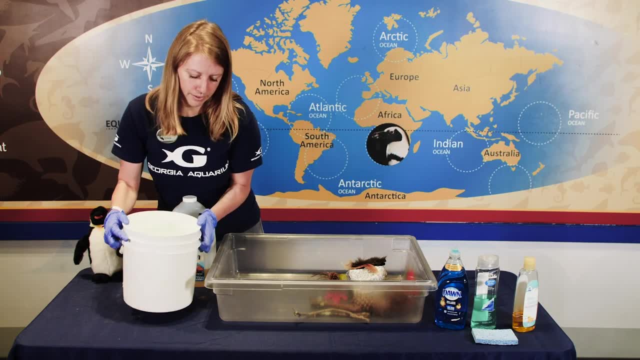 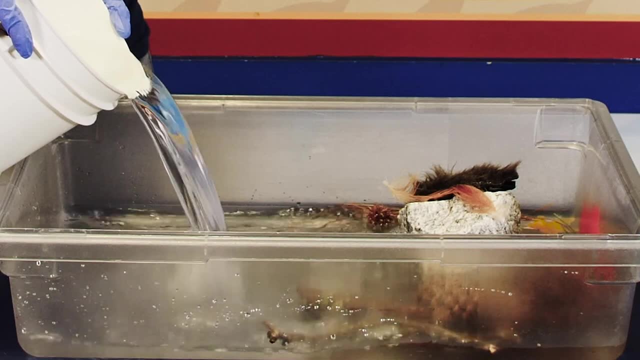 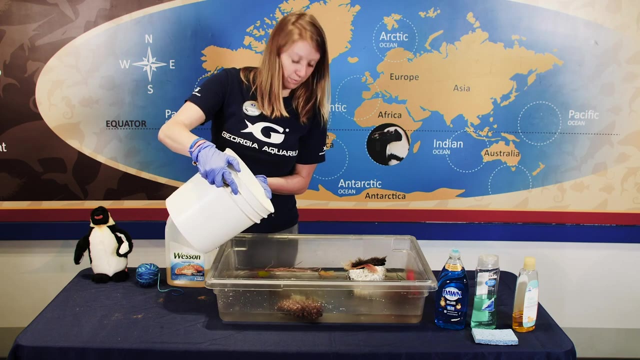 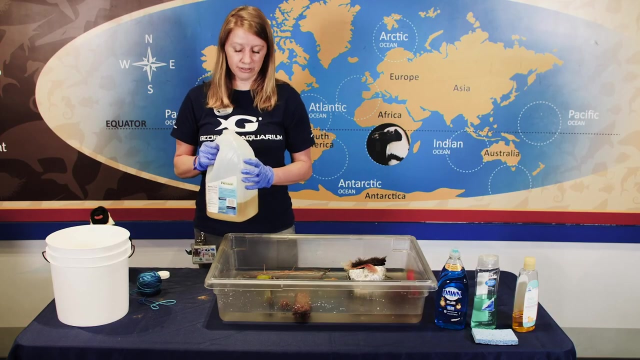 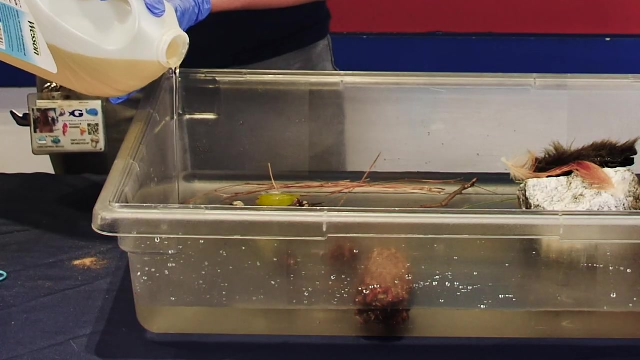 come up to about halfway up to that rock. All right, so here we go. we're going to add our water. Perfect. The last step is adding our oil. You don't need too much oil, and I'll show you about how much to pour in. So here we go. Now, the oil spill does usually occur pretty far offshore, so that's why. 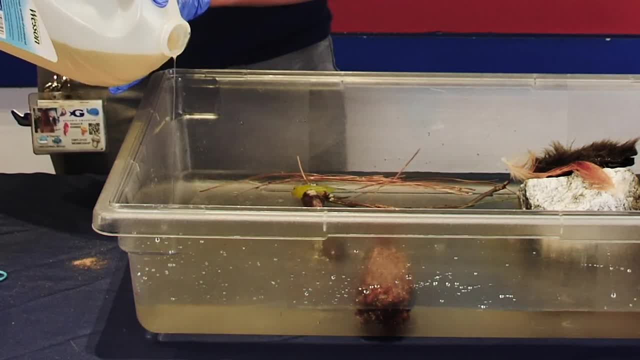 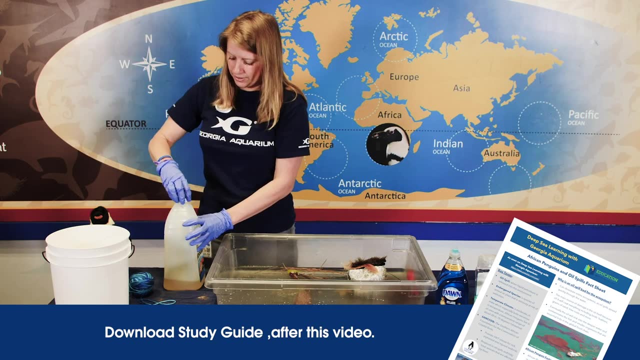 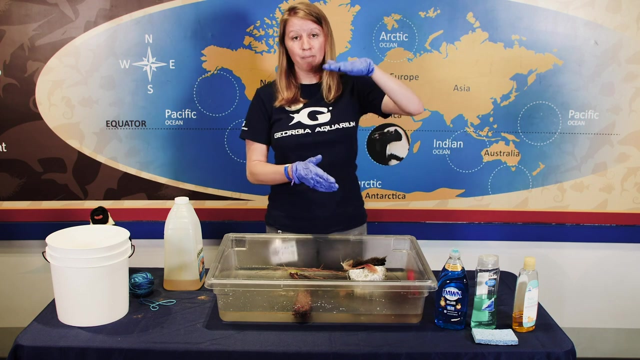 I'm pouring it on the far side of this bin and we're going to see just how long it takes for it to reach the coastline. All right, As I mentioned earlier, before I started the activity, what happens to petroleum in the water? at first is it remains at the surface. Now, after weeks, after the oil spill, petroleum will actually. 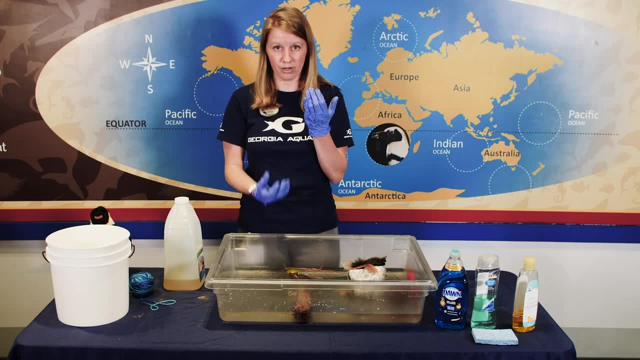 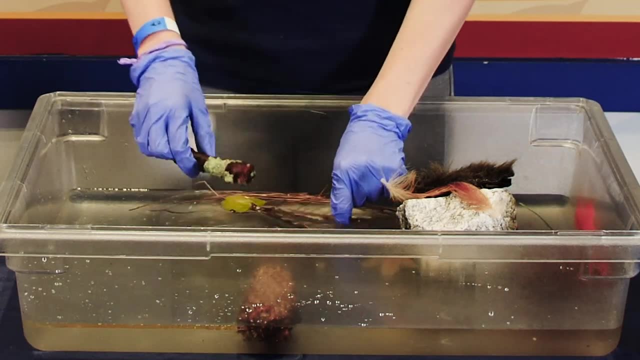 sink down into the water column, affecting all of the water column and marine life in the ocean. Now all you have to do now is kind of wait for that oil to reach the coastline. My sticks and my pine cone are kind of acting as a barrier. That's why it's better to have the biggest. 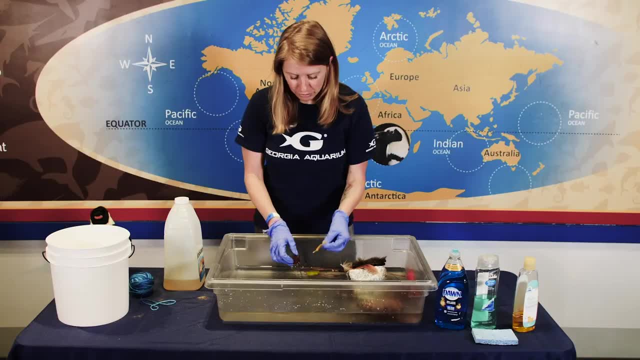 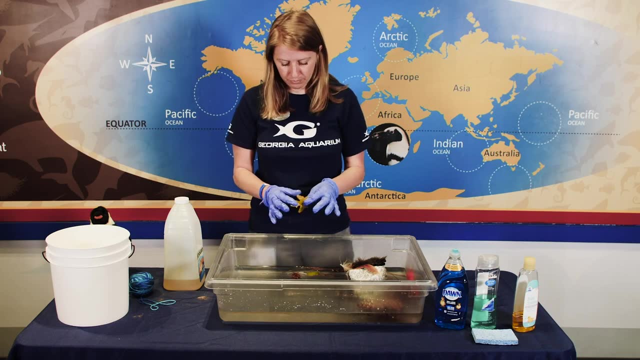 rock you can find for your island. So the first thing I'm going to ask everyone to do is just reach in and kind of feel how the oil is affecting the different materials, materials you have in the water. So we're going to reach in and just kind of feel our stick so you can see they're absolutely 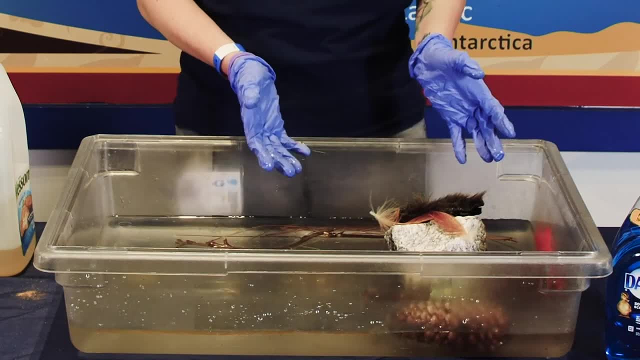 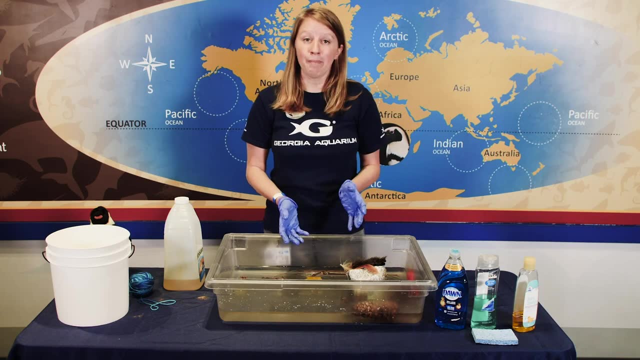 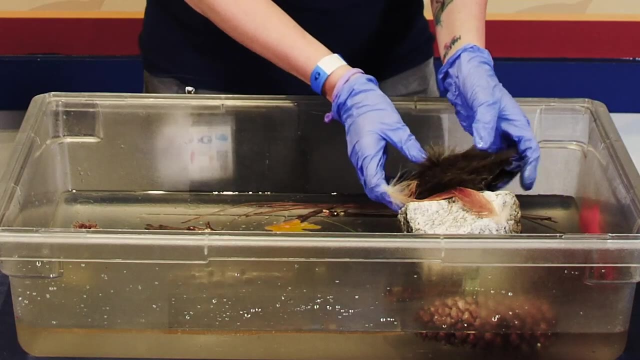 covered with oil, But luckily, because we didn't have enough or have all the water, the fur and the feather did remain safe on the island. Now what would happen, though, is those birds and those safe animals will come to the water because they don't know. it's not an unsafe environment, So what we can. 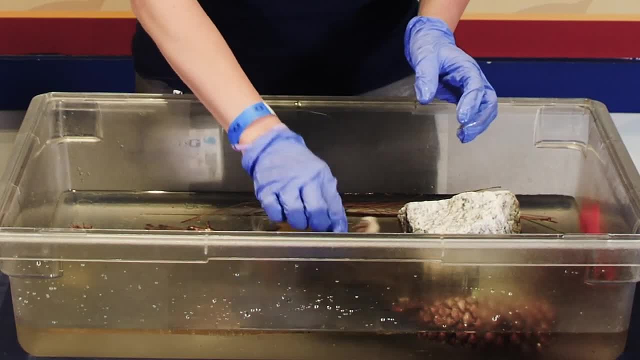 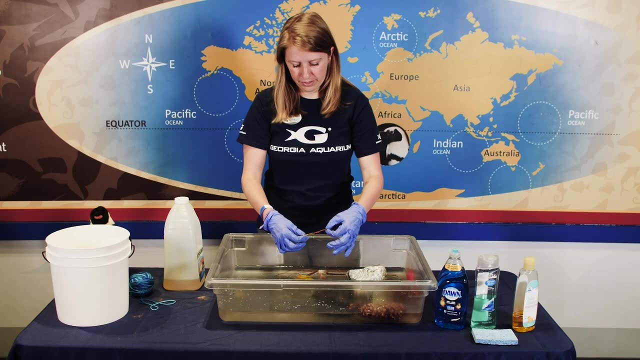 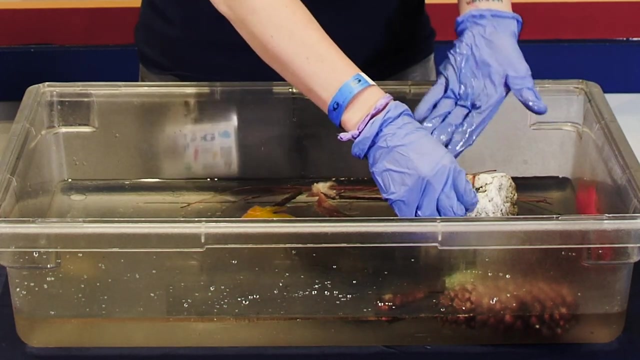 do is we can put our fur and our feathers in the water and we're going to see how that oil affects each of them. All right, so you can see just how much this feather is coated with oil, and this is exactly what happens to marine birds such as African penguins. Now, this is the same thing. 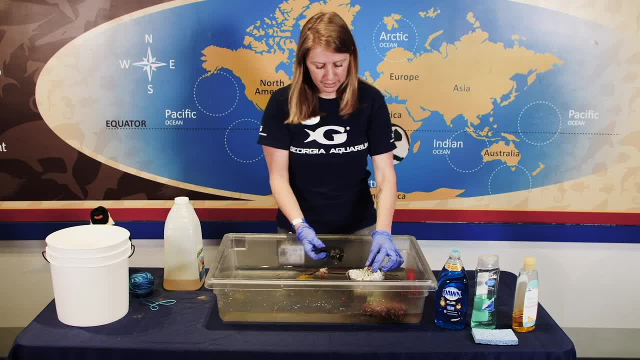 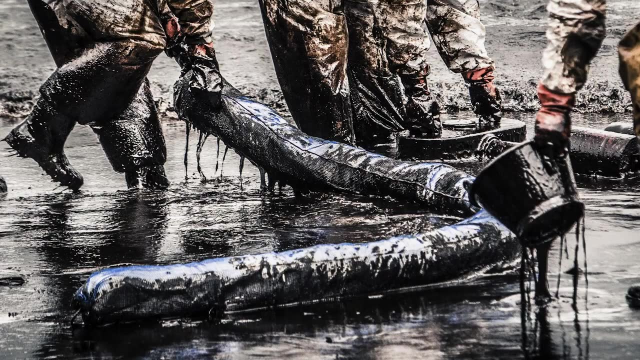 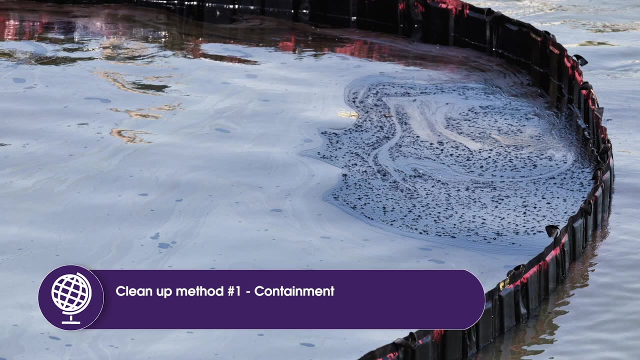 with our fur here, It's absolutely coated with oil. Now the next part of our activity is we're actually going to move to the cleaning and the cleanup side of the activity. Now, in the real world, there's three different types of methods used to clean up oil. The first one is containment. So maybe this string right. we're going to try to. 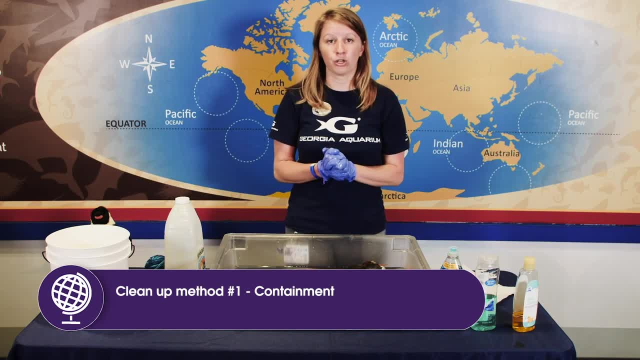 block the oil from hitting the coastline. They use floating barriers, called booms, that actually absorb oil. This doesn't always work perfectly, but it is a type of method they try. The second method is chemical. use chemicals to actually make oil more solid so it's more easily removed. Now the downside to using 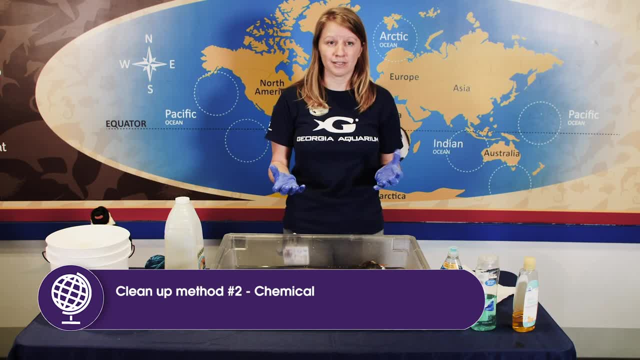 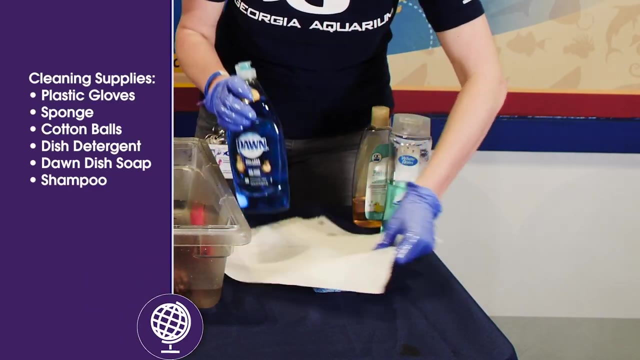 chemicals is you have to add chemicals to marine environments. The third and last way they clean up oil is the one we are going to try, and it's by physically removing the oil. So what we're going to take today is we're actually going to use our Dawn dish soap. get a couple napkins handy. 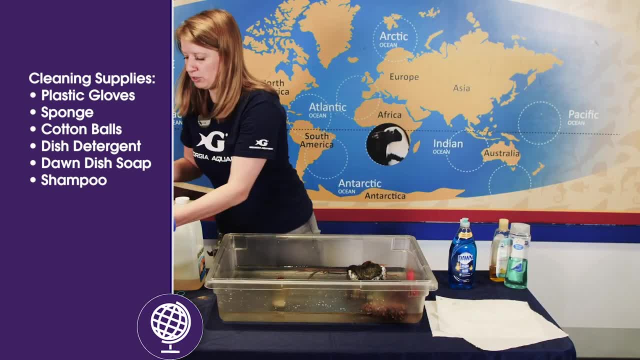 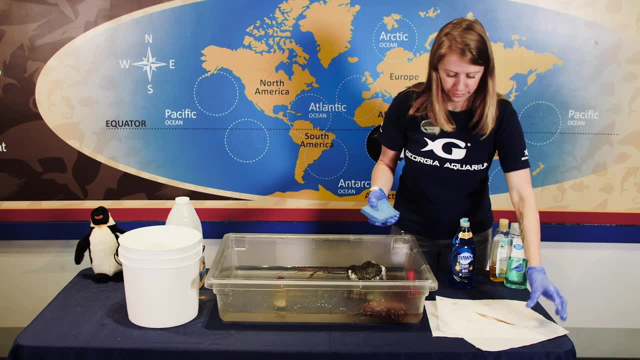 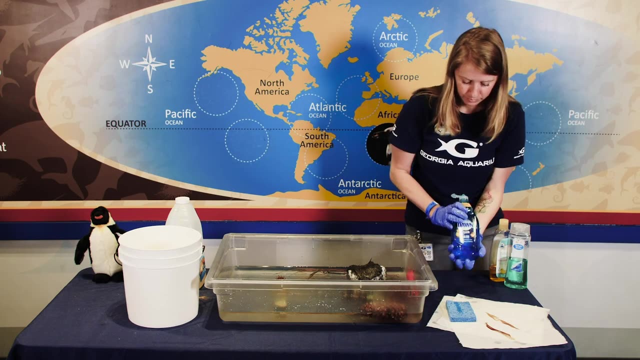 and our sponge. So I left just a little bit of water in this bucket on purpose. Let's try our feathers first. So I have two feathers here that are covered in oil and we're going to add some soap to our sponge. You can see the little birdies on the Dawn dish soap. 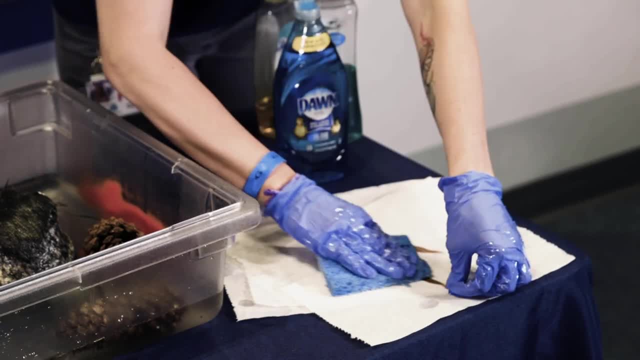 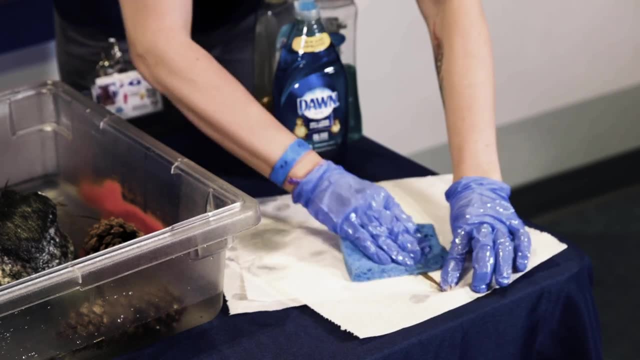 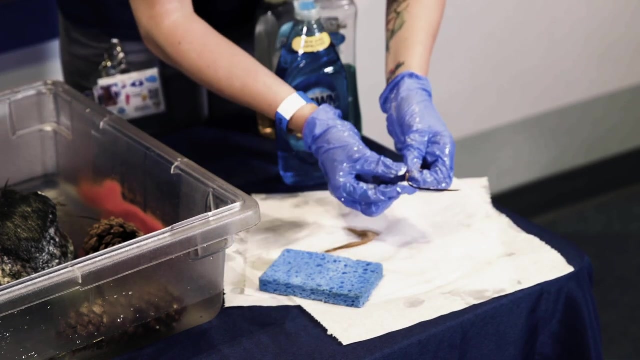 That's what it's advertised for. So this is a physical method of removing oil and this is what people actually do to animals. They are sitting out there and scrubbing their feathers, really trying to remove that oil from them. It takes a lot of hard and careful work when you're dealing with live animals. 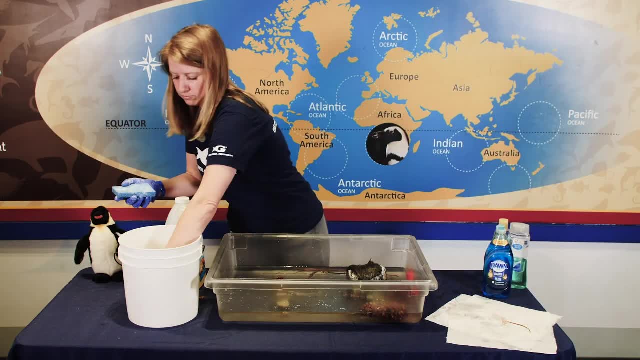 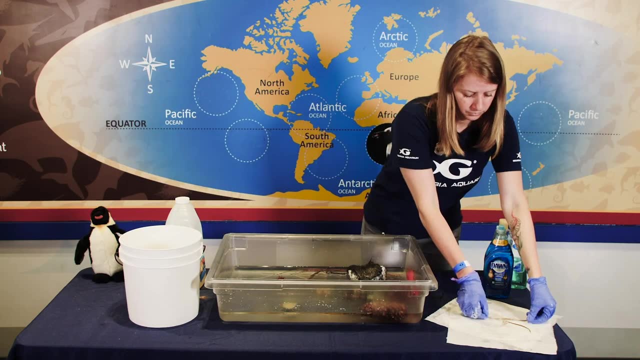 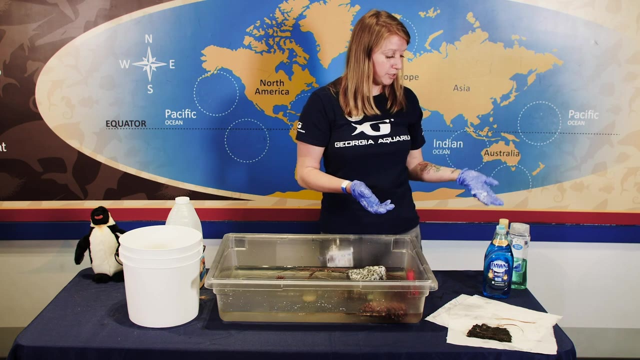 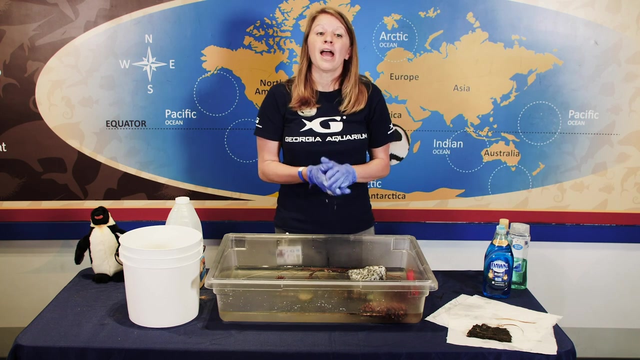 that have been affected by oil, Trying to get some water on it- example of a cleaning technique at home. i encourage you to try others. try using the shampoo or the dish detergent, even laundry detergent- see what works best. now i'm going to leave it at that for a little while, and after you're done, there's a couple things i want you to. 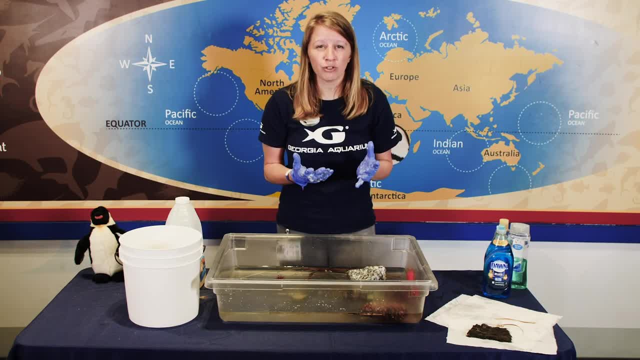 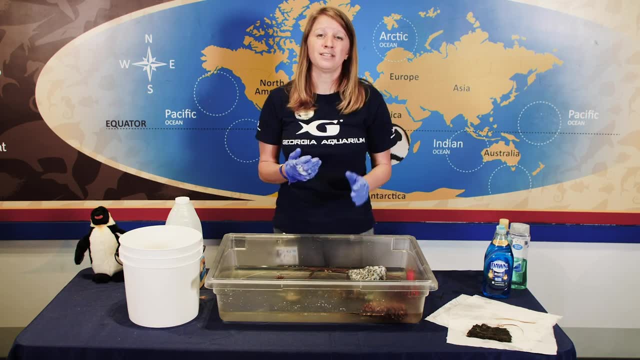 think of after you finish your own activity. what was the most difficult item to physically remove that oil? was it the fur? was it the feather? maybe try the rock itself? this is something that people in the in the real world have to deal with. it's not just the animals, it's the entire ecosystem.